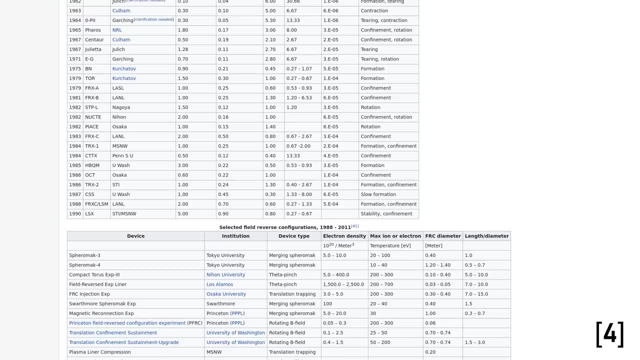 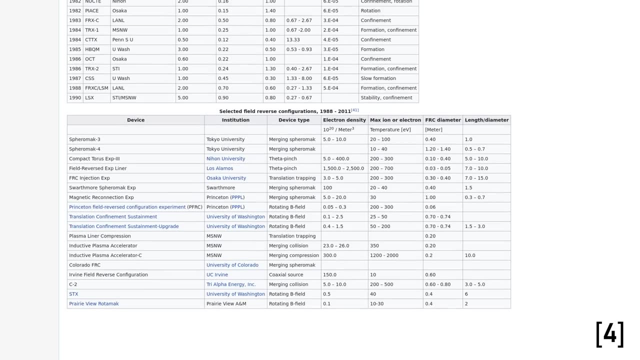 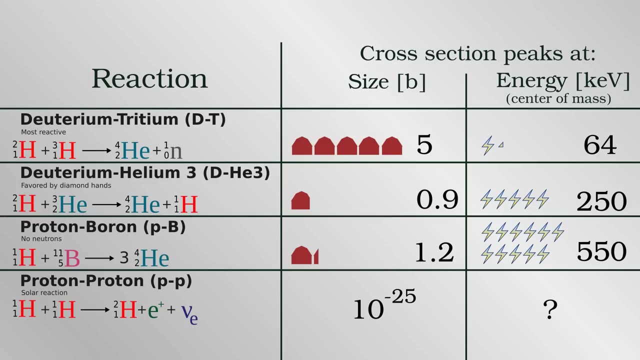 the 1960s, so this is absolutely nothing new, even though CEO David Kirtley said, quote: it's a real, unique version of fusion fuel that Helion and very few others do. end quote: The first challenge for Helion is that they plan on using the deuterium-helium-3 reaction. 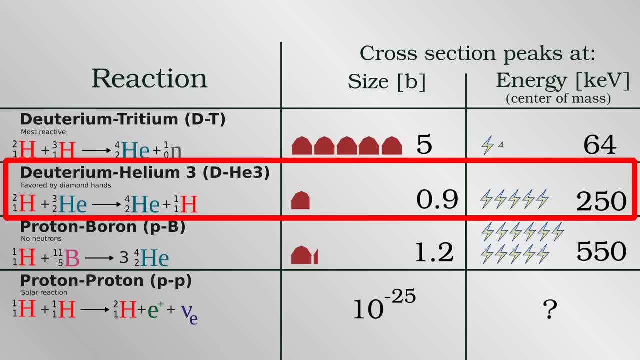 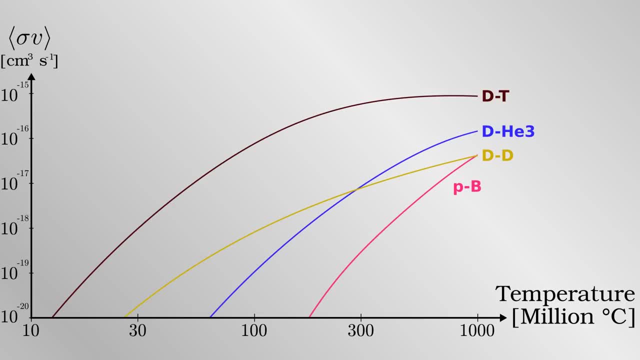 This is a much less reactive fuel mix than deuterium-tritium, which is the reaction in most other approaches. As I said previously, suppose we achieved good power output from a deuterium-tritium reactor. The tritium is a. 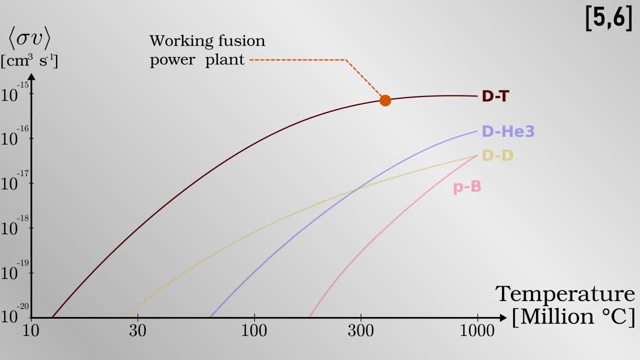 problem because it's hard to make and it gives off neutrons. So we decide to replace the fuel with a deuterium-helium-3 mix instead. This will absolutely clobber our power output. when running at the same temperature as before, We could claw. 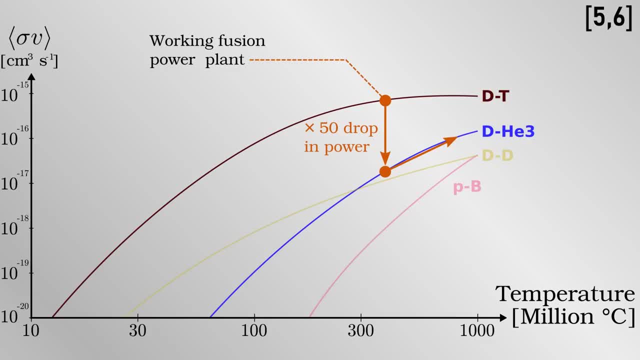 back some of that power if we up the temperature or density, but of course this increases the physics and engineering challenges. Note that in this case some neutrons would still be produced as deuterium nuclei would fuse with each other. In this plot on the x-axis is the temperature in millions of degrees. 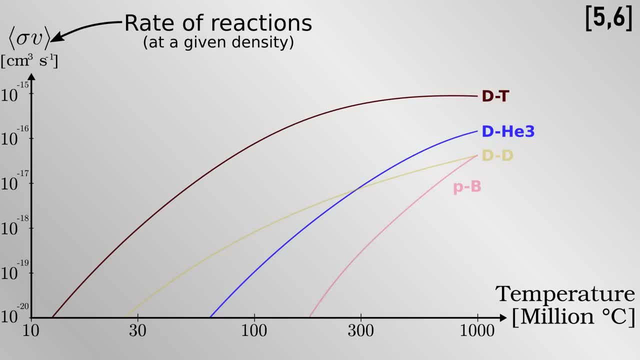 and on the y-axis is the reactivity. I assumed that any commercial reactor would target at least 300 million degrees, but helium seems to be satisfied to have reached 100 million At this temperature. they are 1000 times less reactive than they could be if they went with. 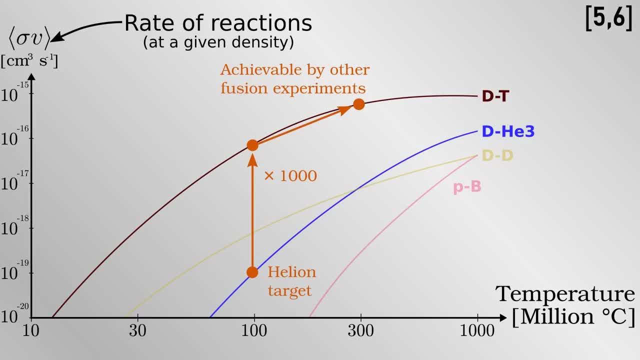 a tritium option, or 5000 times less reactive than a machine like JET at its operational temperatures. It is therefore extremely doubtful to me that they will ever generate energy gain. But hey, maybe venture capitalist funding gives you some sort of magic that will overcome the. 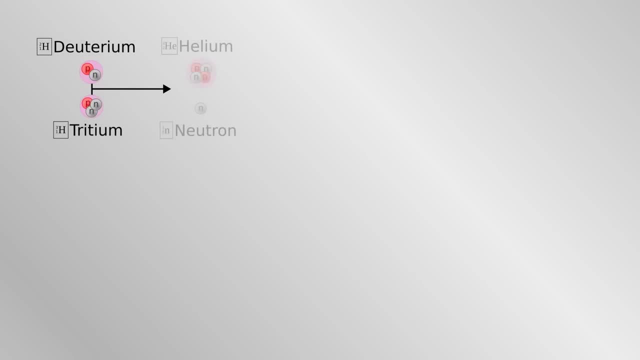 slower reactivity. somehow I did have a chuckle at how real engineering is wrong in their explanation of neutrons in the deuterium-tritium reaction, as if breeding tritium somehow loses the energy carried by the neutron. Also the wording implying that tokamaks can only use. deuterium-tritium was wrong. They could, and sometimes do, have helium-3 fusion. It's just that the plan in future is to use tritium for the previously stated reactivity reasons. The other problem with deuterium-helium-3: 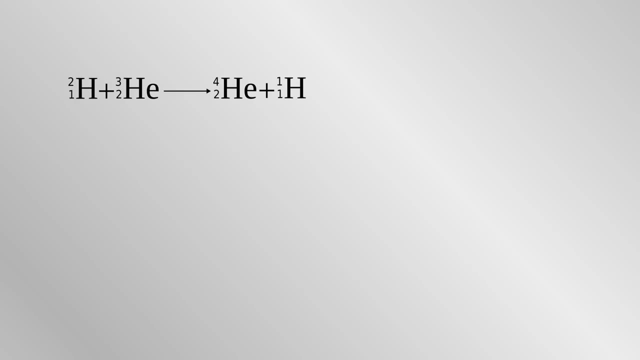 is the extreme amount of radiation which would be put out Now. granted, this reaction itself doesn't involve any radioactive materials whatsoever. However, if you have a mix of these two isotopes, at thermonuclear temperatures, pairs of deuterium nuclei will react with themselves and release neutrons. 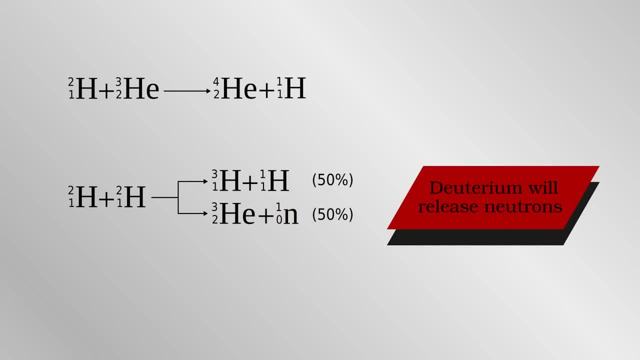 This is a factor which the real engineering video completely ignores, as if you could have a stern talk to the deuterium nuclei and order them to only react with helium and not with each other. Statistically, the chance that two deuteriums react is half of deuterium-helium-3,. 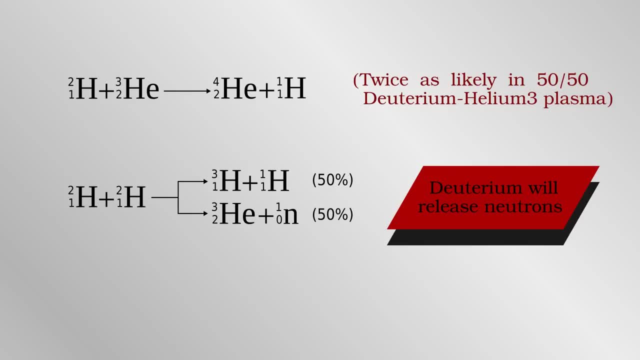 and only half of the former reactions will produce a neutron directly. This means at equal reactivity, one neutron is released for every four deuterium-helium-3 reactions. However, if you look back at the plot I showed before, at 100 million degrees, 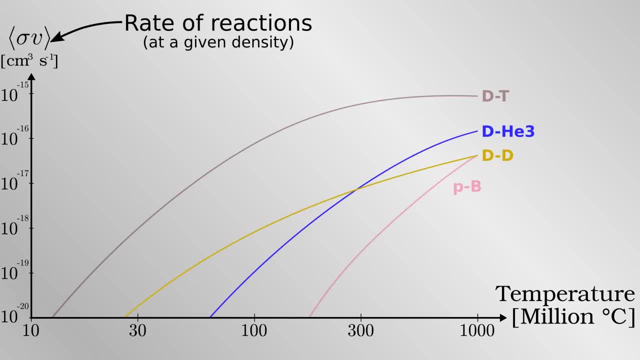 the deuterium-deuterium, reactivity is 7 times higher than deuterium-helium-3.. you are therefore going to get a lot of neutrons when trying to react with helium-3.. to actually produce electrical power, A neutron is about 10 times more deadly than a similar gamma. 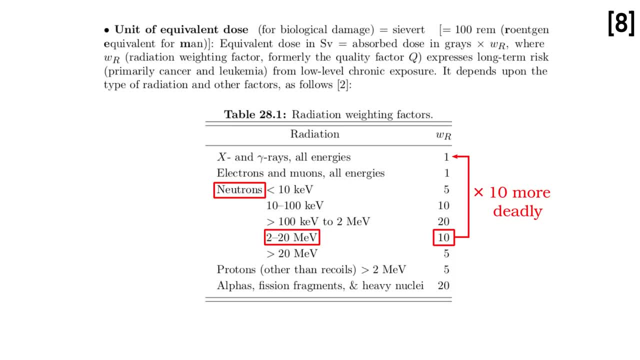 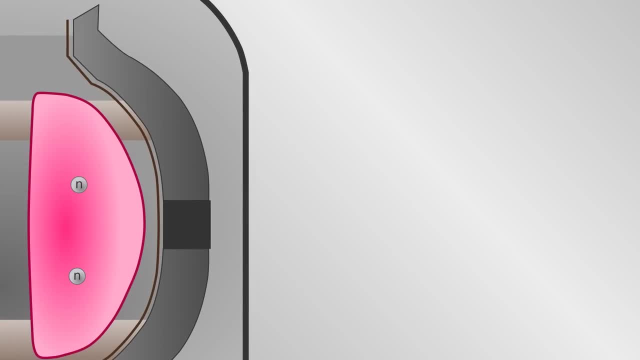 ray and unlike gamma rays, the neutrons will make other things radioactive. after the machine is switched off, as I said previously, You must physically have roughly a meter of dense material around your fusion reactor. Because the neutrons are not charged, they are not slowed down unless 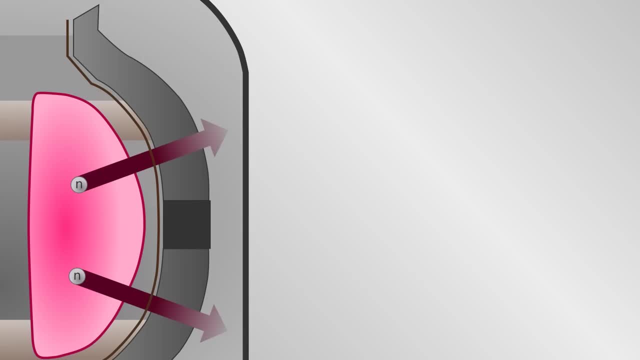 they interact with a nucleus directly. You must therefore put enough atoms in their way to stop them. When a neutron is absorbed by any element other than lithium or beryllium, it will typically turn the stable nucleus into a heavier radioactive one. If the phosphorus in your DNA absorbs a 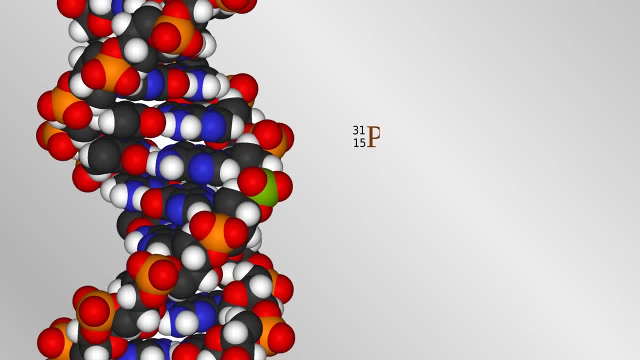 neutron, it will turn into an unstable isotope, which will then decay by means of beta emission and become a sulfur atom. I hope I don't need to say this, but both of these things are very bad for your DNA Helium. do not have a meter of solid material around their reactor to attenuate. 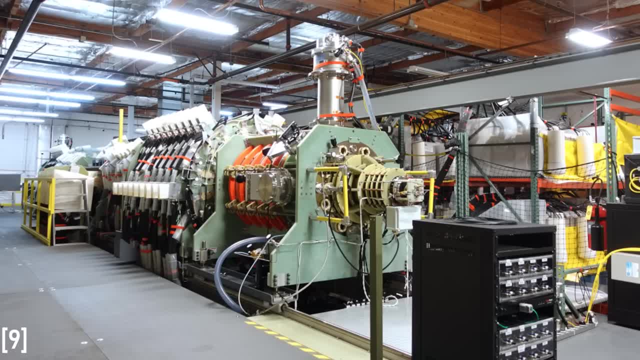 neutrons. If the Trenter machine, as picked up in the video, has a neutron in its reactor, it will have a neutron in its reactor. If the Trenter machine, as pictured, were to be producing power plant levels of energy, it would be like the exploded Chernobyl reactor number 4.. This problem is absolutely non-negotiable. If you are producing fusion energy from deuterium-helium-3,, you are generating a lot of corresponding neutrons and making everything radioactive, Even at higher plasma temperatures, where the balance of these two reactions I talked about is more favourable. towards the helium one. you would still be at dangerous neutron levels, Even if everything goes as planned. you would still be at dangerous neutron levels. Even if everything goes as planned, they will need a nuclear rated facility, radiation shielding, a tritium separation plant.